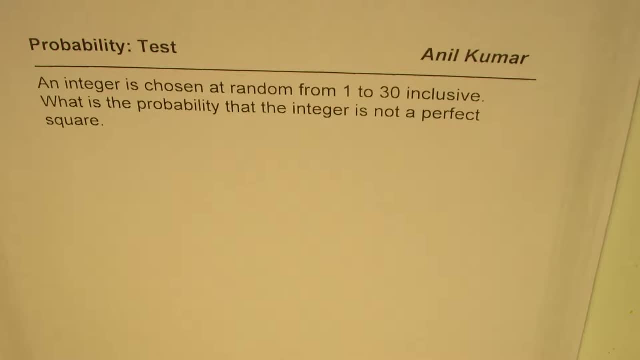 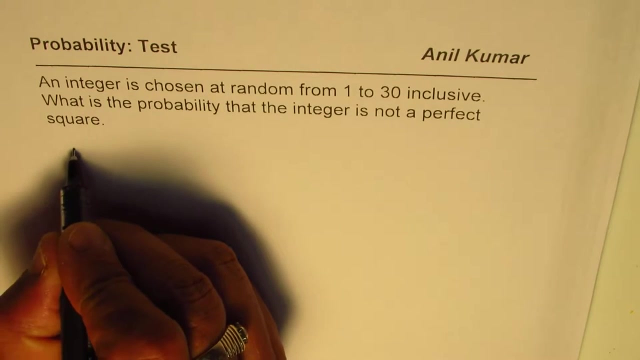 I am Anil Kumar. I have taken a few questions to review so that we can prepare for our test on probability. The question here is: an integer is chosen at random from 1 to 30, inclusive right. So 1 and 30 are included. What is the probability that the integer is not a perfect square? So here in a sample space, how many elements are there? Numbers from 1 to 30 makes it. 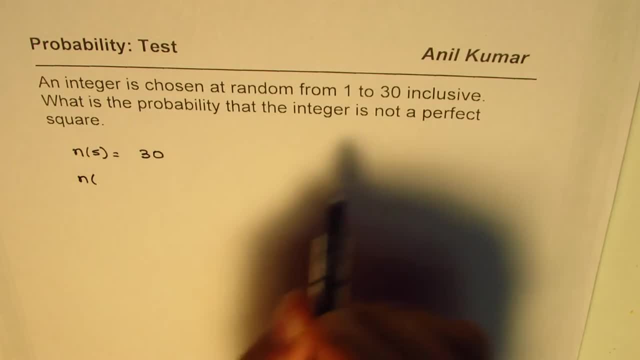 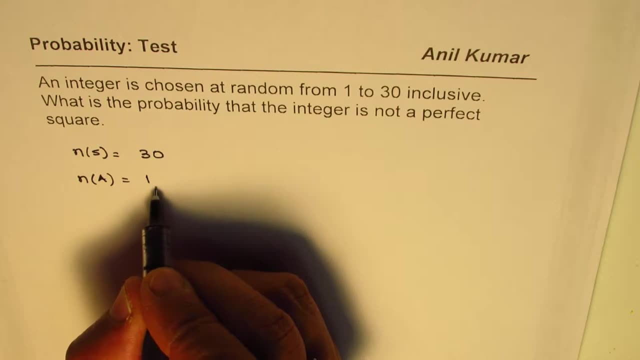 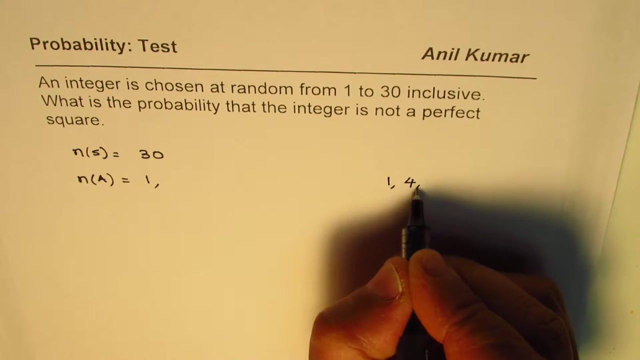 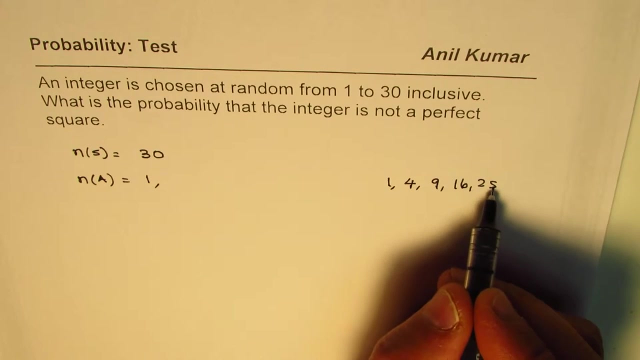 30, right. Now we need to find how many numbers are perfect squares within this. So numbers which are perfect square are: 1 square is 1, 2 square. I should actually write here: 1 square is 1, 2 square is 4, 3 square is 9, 4 square is 16, 5 square is 25.. So numbers are 1,, 2,, 3,, 4, 5, right, So we have 5 numbers which are perfect. 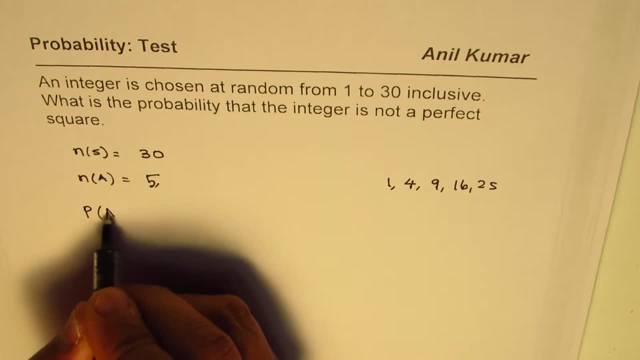 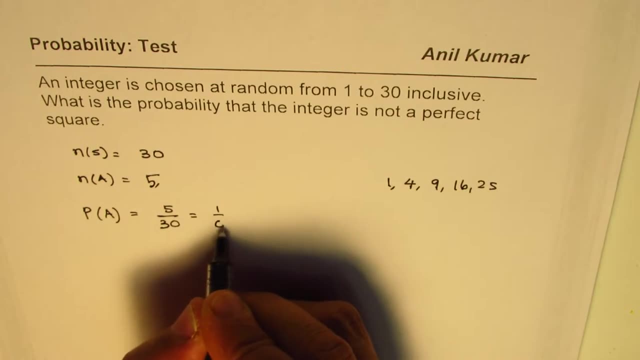 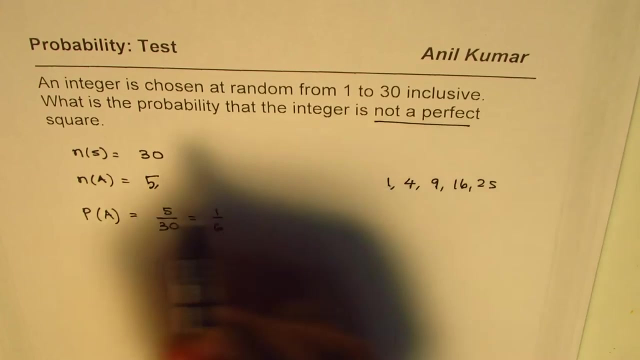 squares and therefore the probability of event A is 5 out of 30, correct So, which could be simplified as 1 over 6.. Now, as a practice question, you can change the question to not a perfect square, to not a perfect cube, okay, So here the question is an integer. 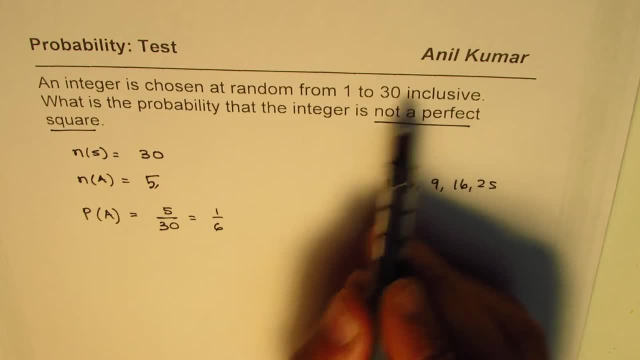 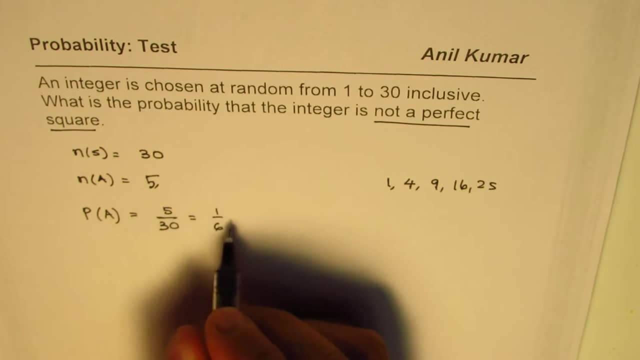 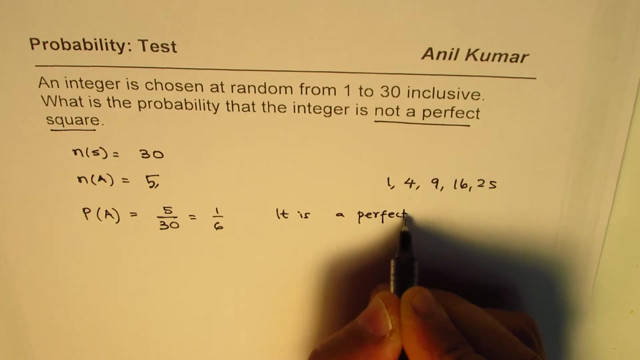 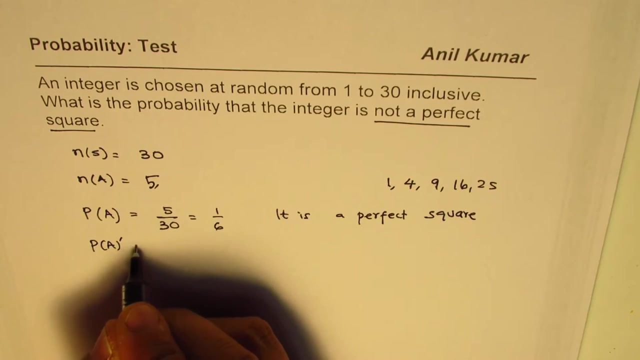 is chosen at random from 1 to 30, inclusive. What is the probability that integer is not not a perfect square? well, this is the problem: probability where it is a perfect square. so this is: it is a perfect square. right, this is what we found. we need not a perfect square, so we need complement of this. that should be. 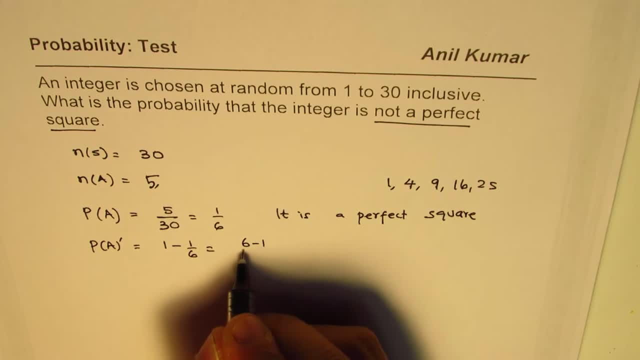 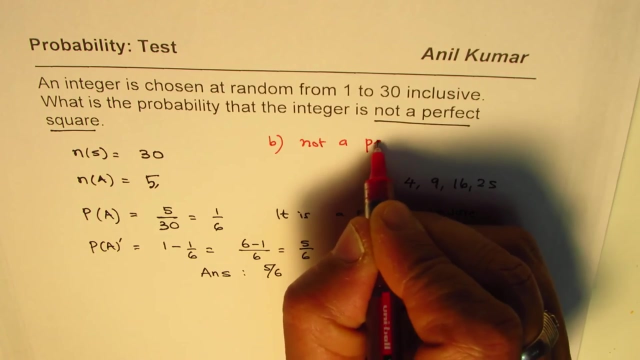 1 minus 1 over 6, that is, 6 minus 1 over 6 or 5 over 6, right? so our answer is: the probability is 5 over 6, for the number not being a perfect square. right now, let me change this question. let let's say: question, for you is not a perfect cube. 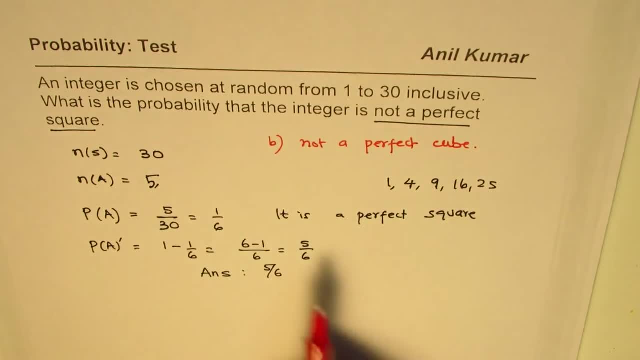 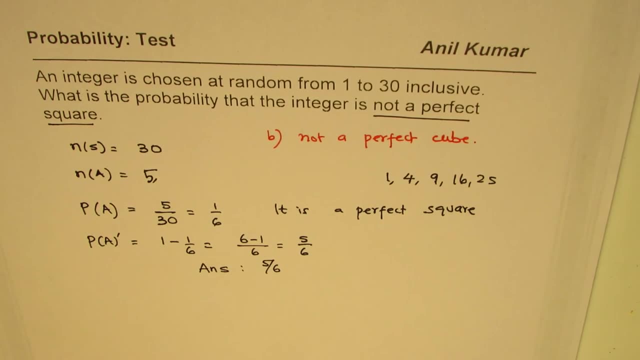 okay, so we just change this question, so do this question now you can adopt the same method. I'm Anil Kumar. I hope that helps. thank you and all the best.